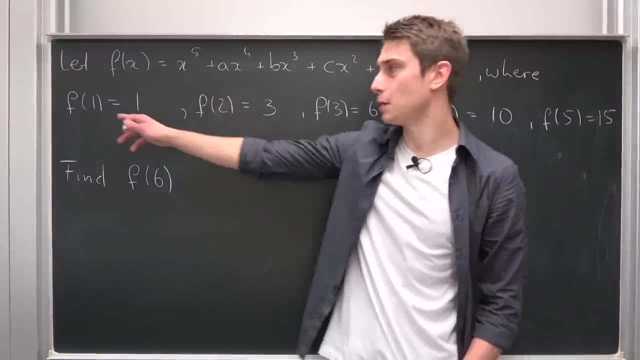 And also we have some initial values for this polynomial up here, namely f of 1 is 1,, f of 2 is 3, blah, blah, blah, And our main goal for today is to find out f of 6.. 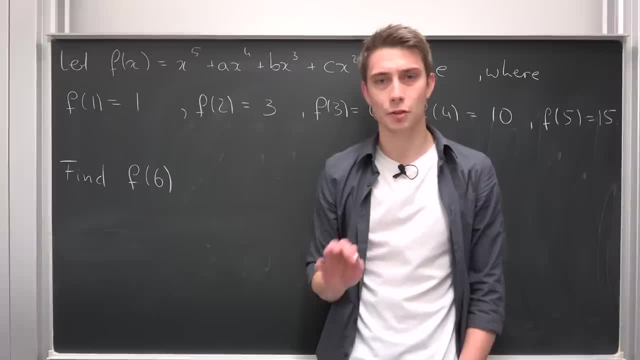 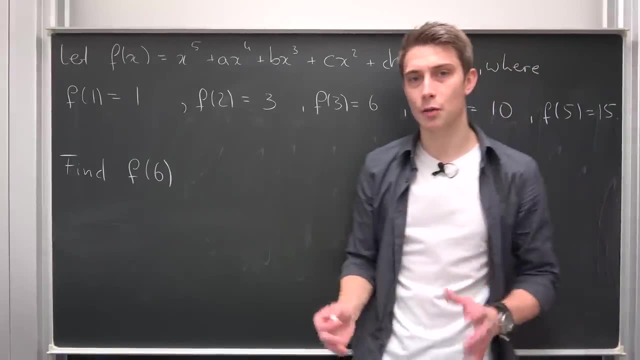 How would you go on with this? Well, there's a strategy you might have seen before. It's often used in algebra. actually, What you want to do, we want to construct ourselves a new polynomial where those initial values right here are going to be our roots. 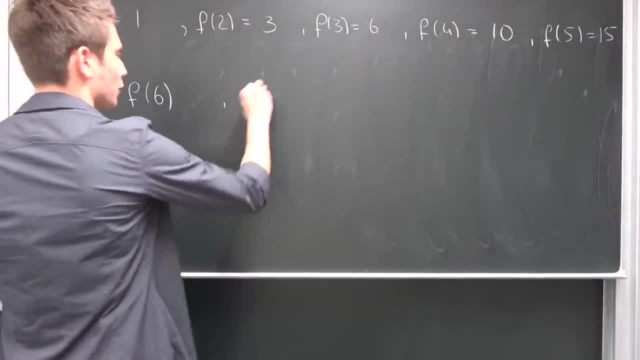 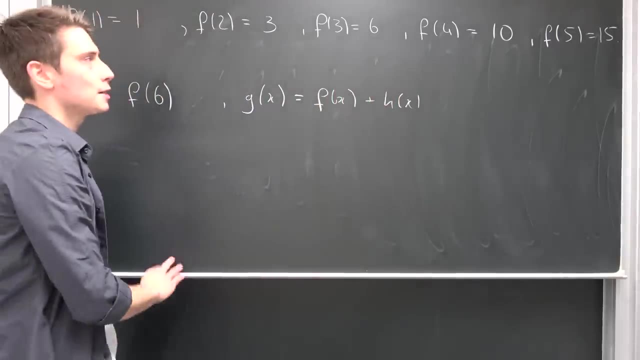 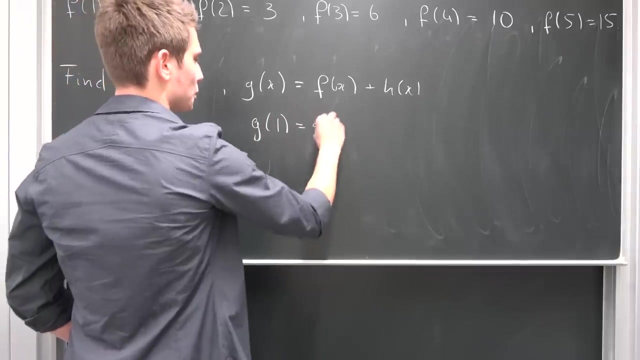 Meaning. we want to find out, for example, some g of x being equal to, well, f of x plus some unknown h of x, such that those are our roots, So such that g of 1 is equal to, g of 2 is equal to, blah, blah, blah. 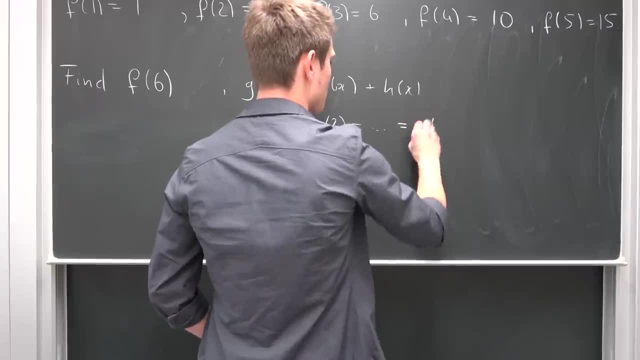 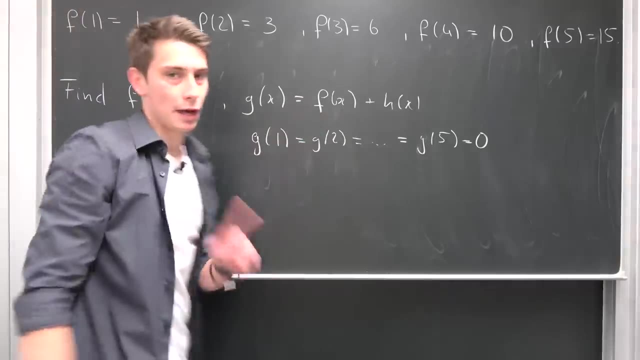 It's going to be equal to f of 5, g of 5,, I'm sorry, being equal to 0. Such that we can factor this thing right here to find out our f of x in the end. So this is a strategy you might have seen before. 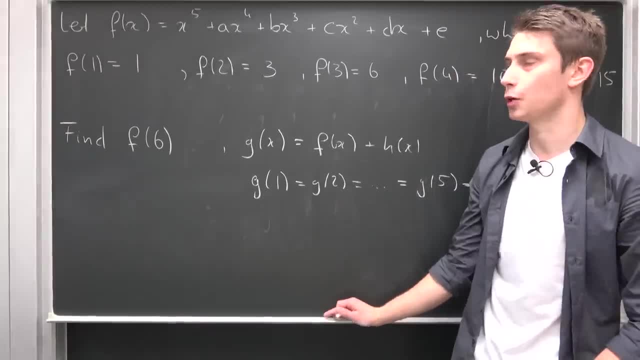 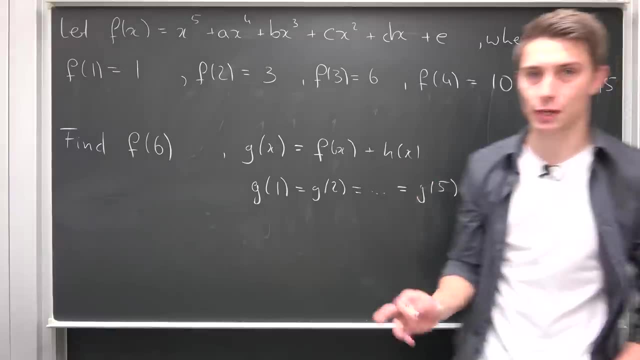 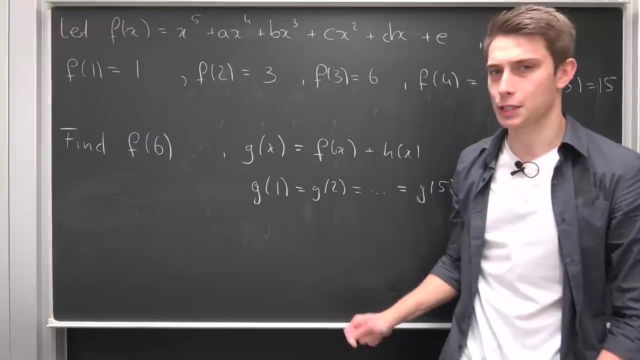 It's often used in algebra, in abstract algebra. Okay, How would you go on with something like this? So how can we actually find out our h of x, for example? Maybe you can see a certain pattern in here. I'm going to draw a little bit and maybe you can see it from there. 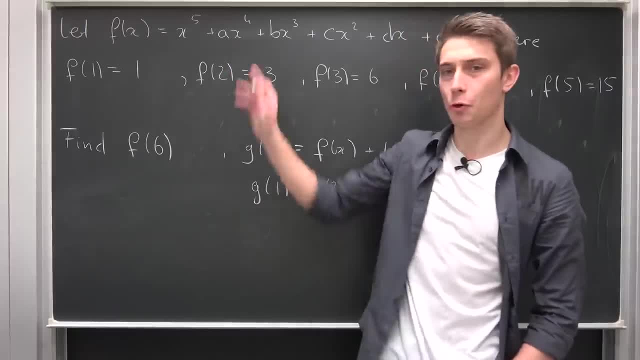 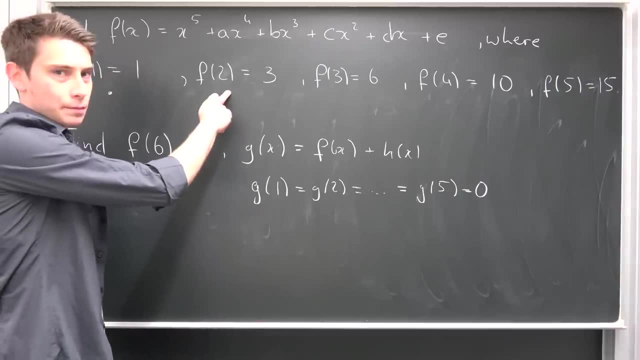 f of 1 is equal to 1.. Let's interpret our polynomial as just little dots. So f of 1 is equal to 1.. Okay, first dot. f of 2 is equal to 3.. Why not interpret this x value we have plugged in as the number of rows? 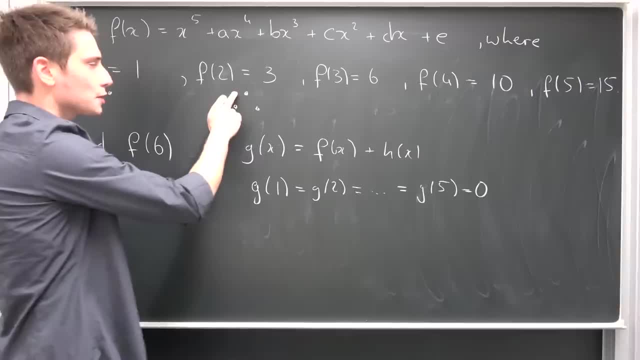 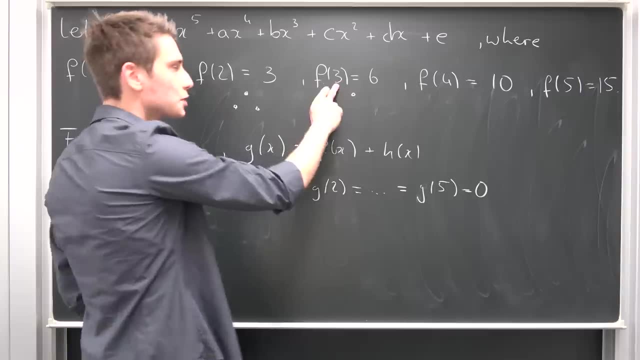 So 1 row gives us 1 dot, 2 rows gives us 3 dots, So 1 plus 2 is 3.. What about the next one? So we have 3 rows, So 1, that's the second row, and then we have our third row. 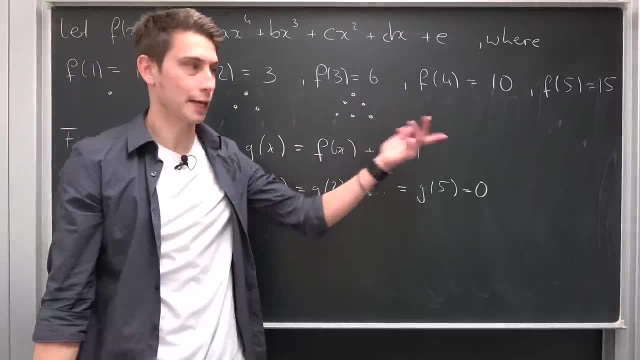 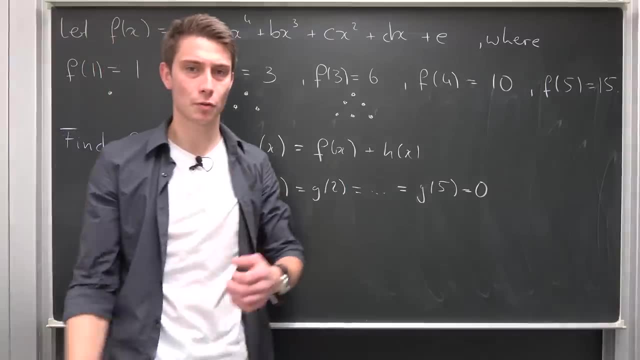 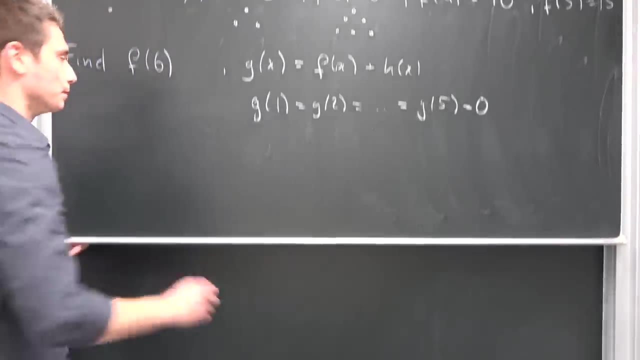 Okay, Maybe you have heard about those before. Those are called triangular numbers, if I remember correctly, But there's another term used for this. This thing right here just follows from the finite summation of natural numbers, one after another. It's called the little Gauss Gauss theorem. 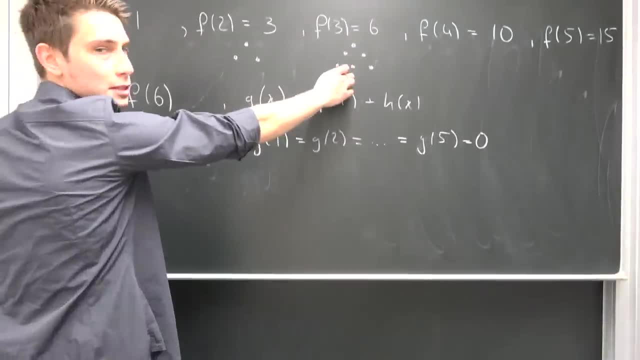 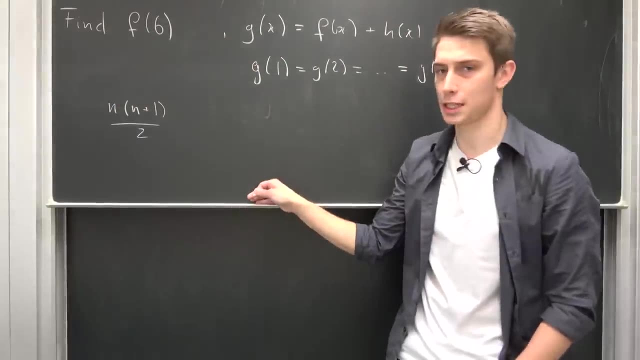 So we can rewrite this right here, the number of dots as nothing but n times n plus 1, over 2.. You can prove by induction that this right here holds. So if you plug in the number 5 right here, this would be that right here. 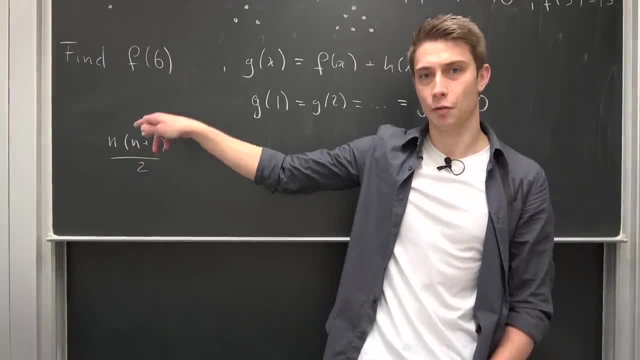 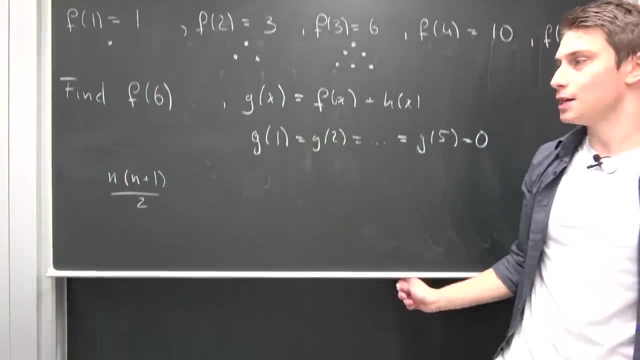 We get 5 squared plus 5,, which is 30, over 2,, which is going to result in 15.. And this is just this right here. And yeah, This is just how this pattern works. on the first five terms. 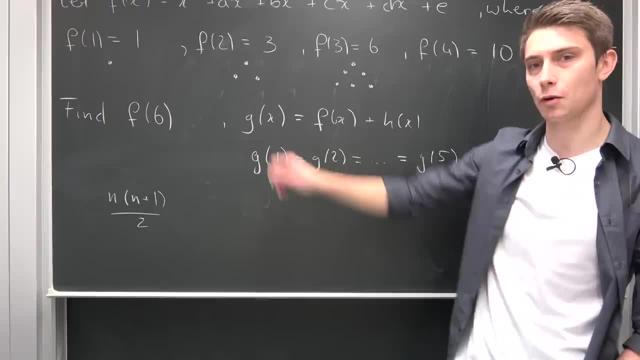 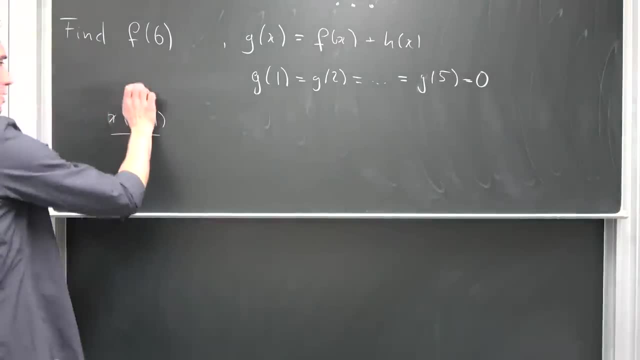 And this is actually really good, because this allows us to construct our g of x right here, Where this right here is our h of x respectively. So if we replace this with an x, this is going to be our h of x. 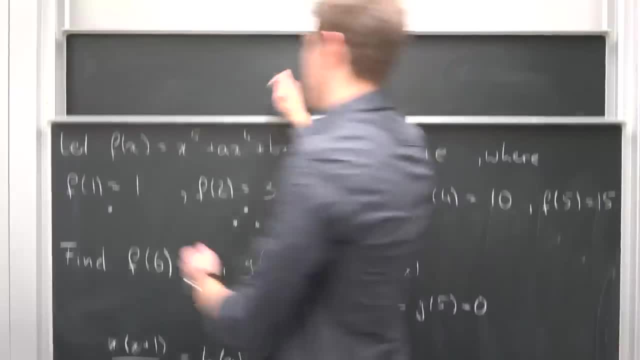 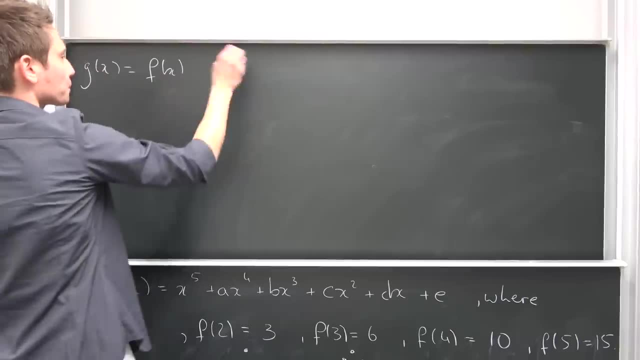 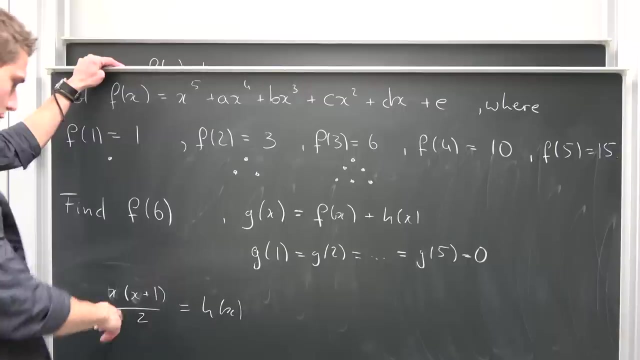 Okay, Now we can plug this into here and see what we actually get. So our g of x is now f of x, Which is still Still unknown, And then positive. Let's put a positive right here at the moment. 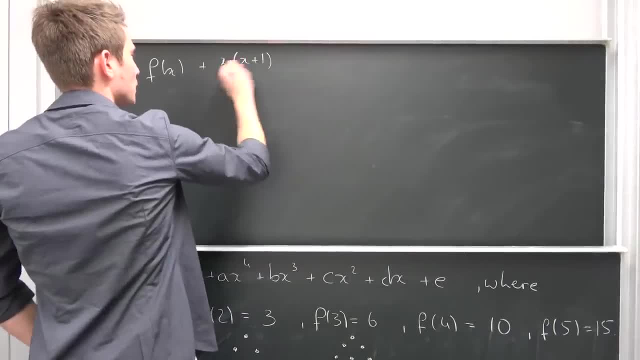 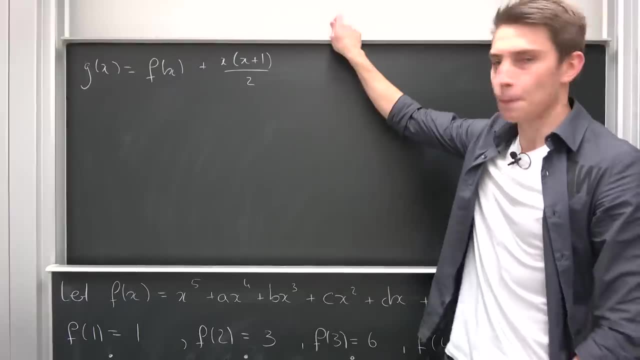 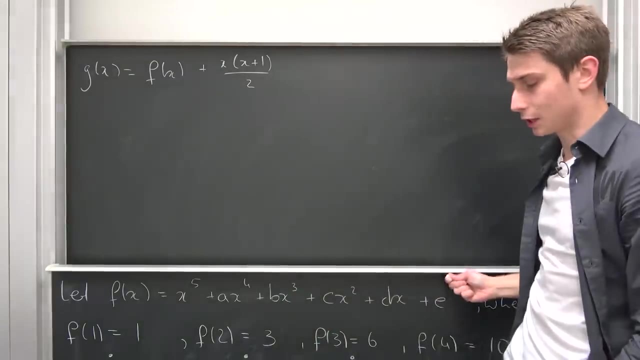 This right here: X times x plus 1, over 2.. Okay, This is just how you can do this. Now you might ask yourself: do we need a positive or negative sign? It really depends on your function that you have right here. 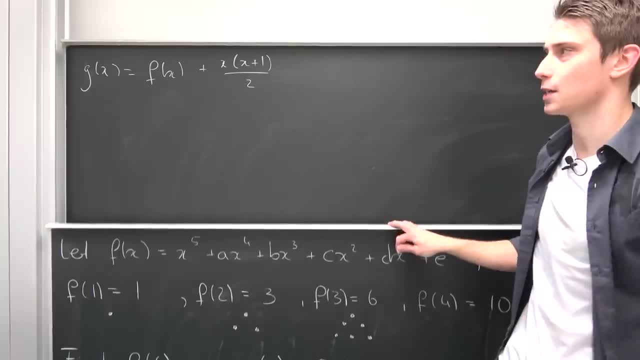 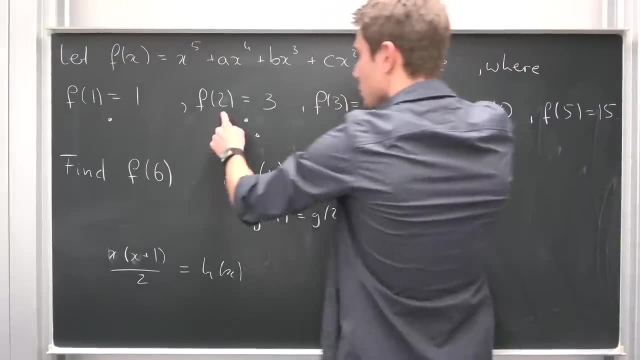 But I would, But I would invite you To place a little negative sign right here, Just because we want those right here to be our root. So all those initial values we have plugged into here in our f are going to be our roots. 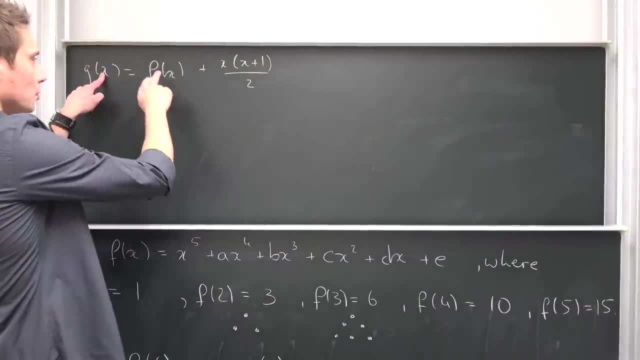 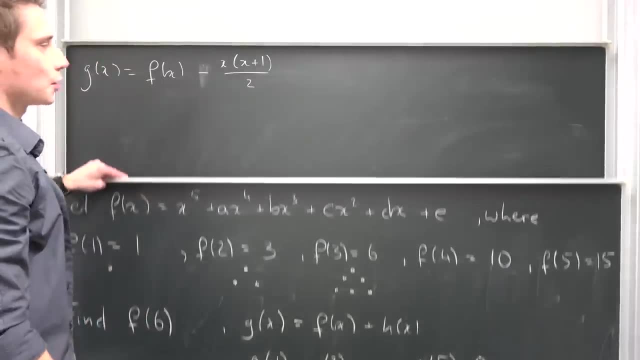 So if we take g of 1,, for example, we get f of 1,, which is 1, and then minus the first triangular number, 1.. So it really depends on your h of x. But I want you guys to notice something. 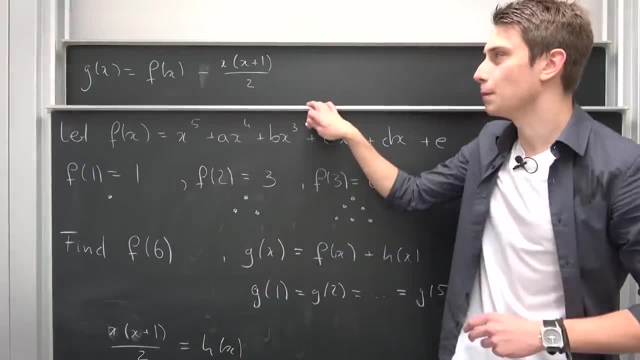 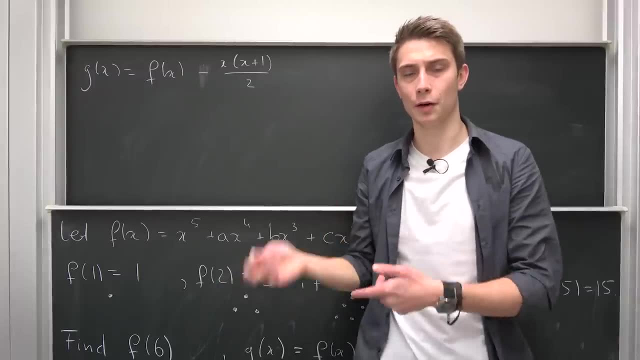 Our f of x is nothing but a fifth-degree monic polynomial. And this right here is nothing but a second-degree polynomial. And if we subtract a fifth-degree from a two-degree polynomial, we are just going to get a fifth-degree polynomial once again. 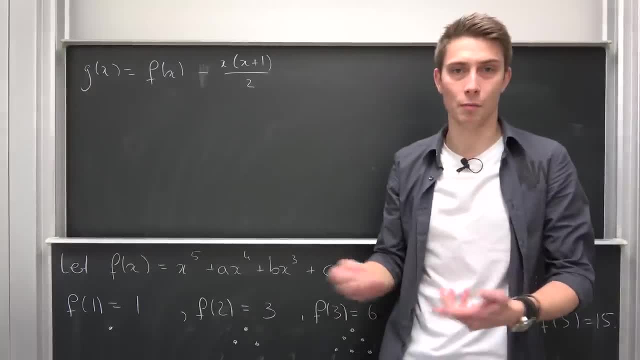 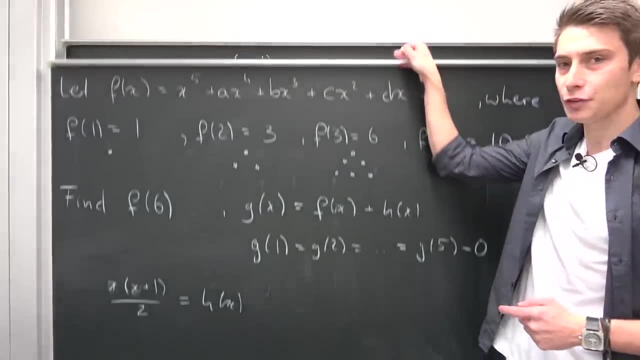 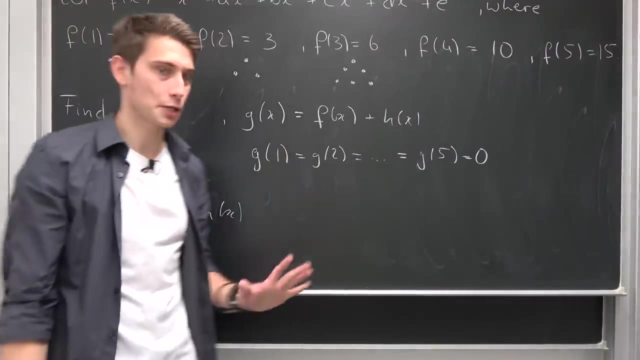 So our g of x is actually just another monic fifth-degree polynomial. But here's the really really cool fact about that: We have a fifth-degree polynomial And this fifth-degree polynomial has exactly five real or complex roots. In this case, they are real roots. 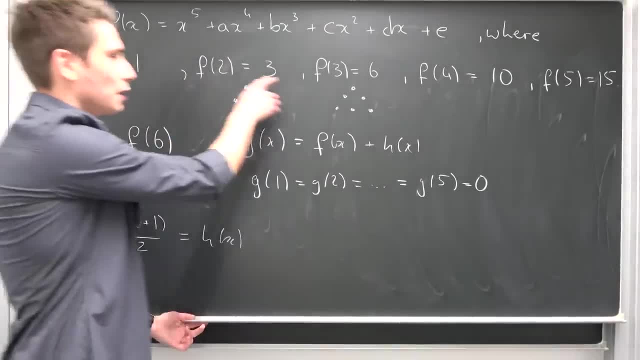 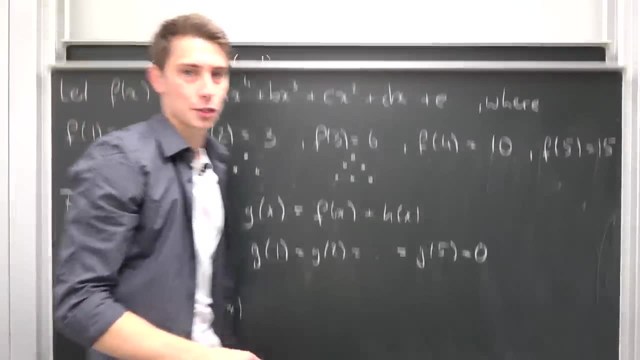 But we have found all of those out because all of our five initial values are just those right here. So you see, we have found out all the roots that our g of x actually has Meaning. this allows us to actually factor our g of x. 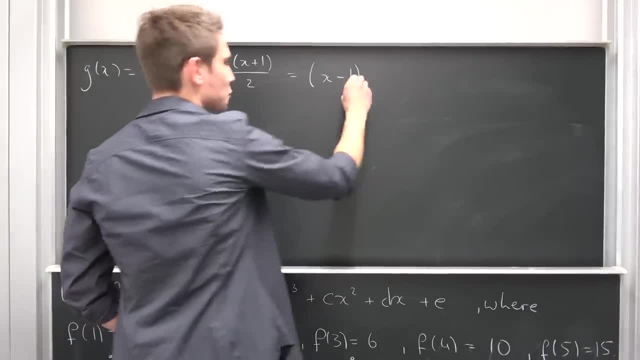 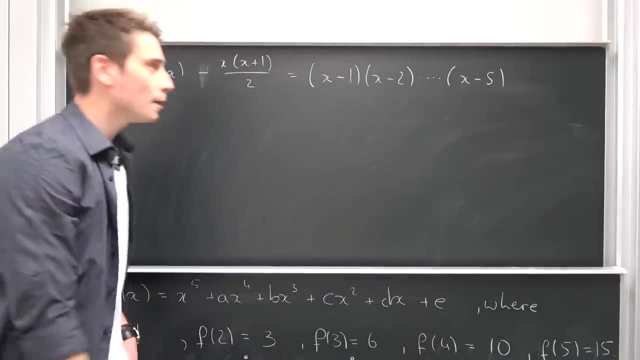 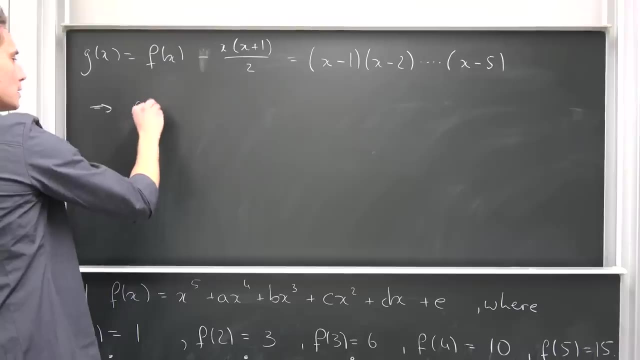 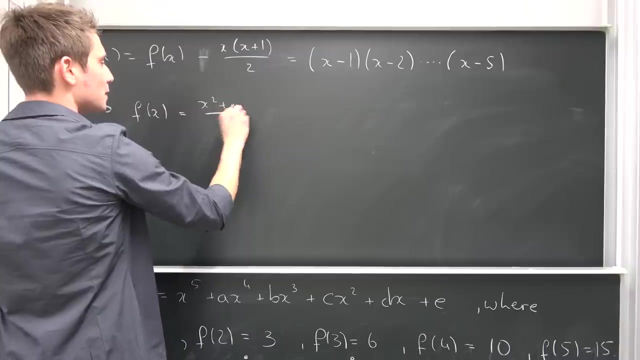 Just simple algebra Meaning: we have x minus the first root, Times x minus the second root, Dot dot dot Until x minus the last root. And this is actually really cool, Because now we can just add this term on both sides, So that we can get f of x being nothing but well x squared plus x over 2 plus x minus 1, dot dot dot x minus 5.. 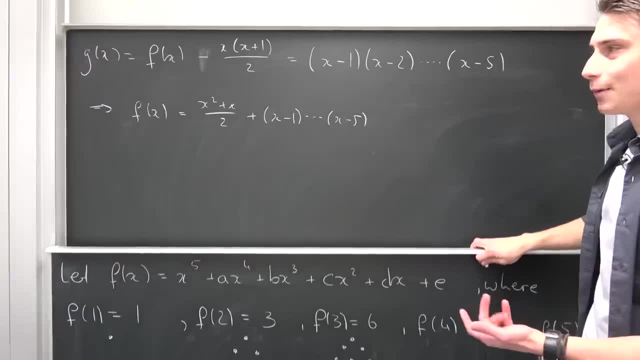 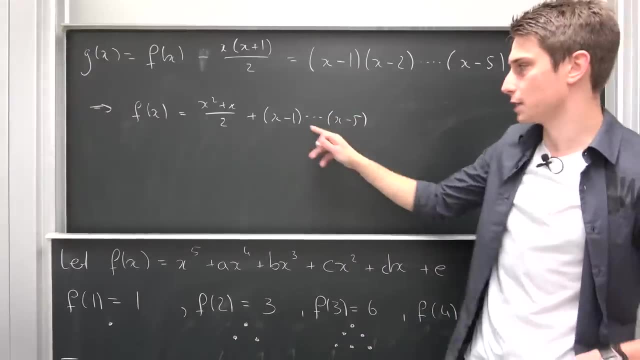 It's as easy as it is, Okay. And well, now we can just plug our 6 into here, because we have found the final definition for our f of x. If we plug 6 into here, this is going to give us 1 times 2 times 3 times, 4 times 5.. 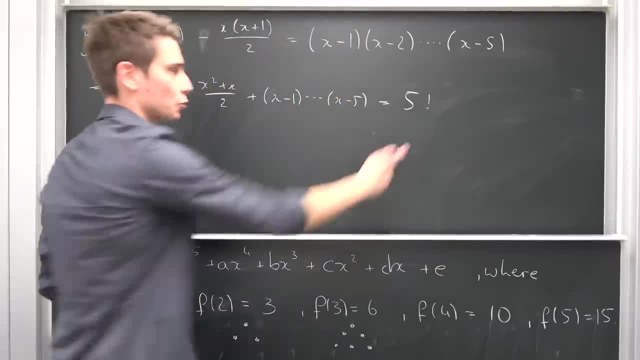 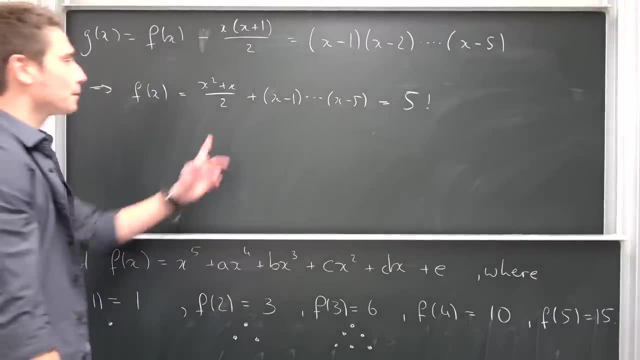 Which is nothing but 5 factorial on this part right here. I'm going to put it here at first, because, well, our addition commutes on the natural entry numbers etc. And if we plug 6 into here, this is nothing but plus 36 plus 6.. 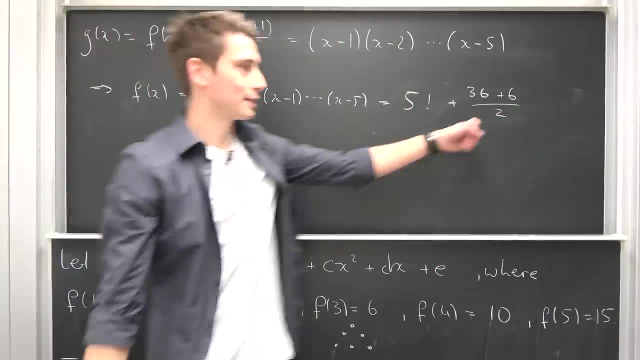 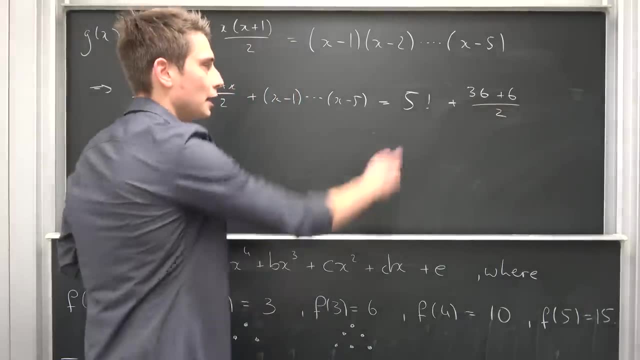 Over 2.. Well, this is really quite easy. This is just going to give us 21 in the end. So this is 18 plus 3, which is 21.. 5 factorial is 24 times 5, 120.. 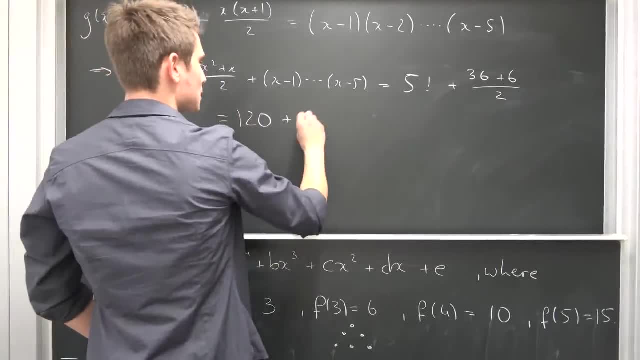 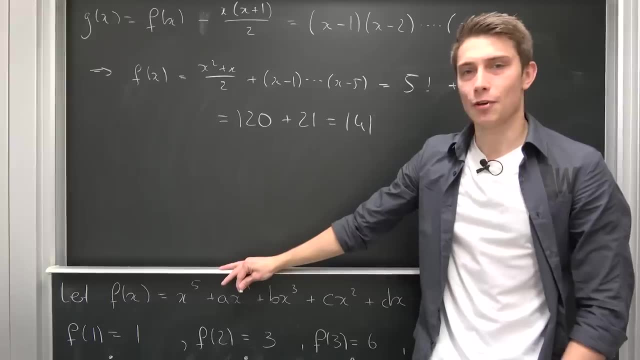 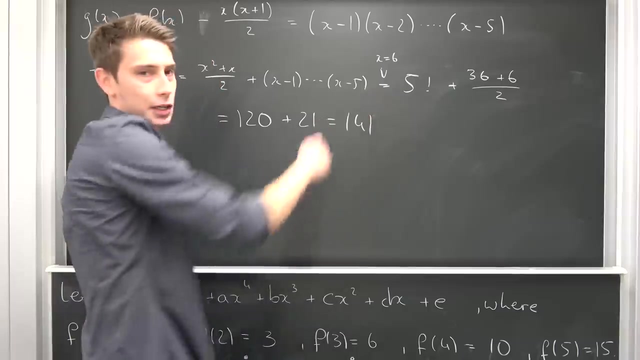 So this is going to give us 120 plus 21,, which is nothing but 141.. And then we are done. So we have found out our f of 6.. So if you plug in x being equal to 6.. So this is not an equal sign.